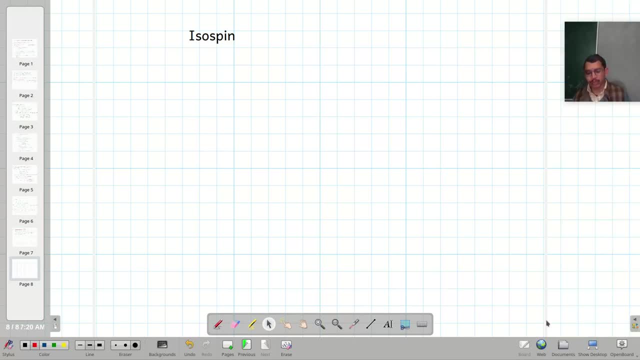 So today I am going to talk about isospin. I divided this lecture into two parts, So in the first part I will talk about concept of spin. First part is where I will talk about concept of spin- Sorry, not spin, but isospin- and in the second part I will talk about the algebra of isospin. 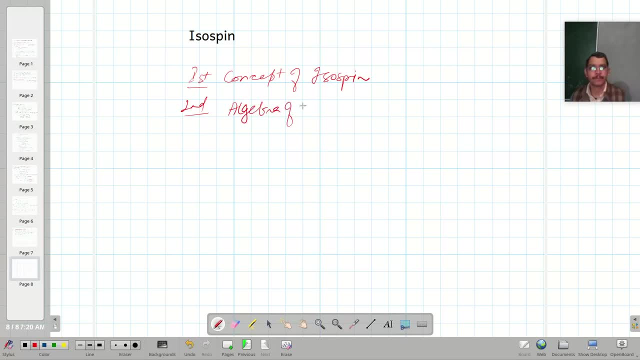 These are the two parts, what which I will talk about in this lecture. So let me talk about that: how the idea of isospin came, So as we know that. so, concept of isospin. So for this, consider the electrons- sorry, consider protons, and 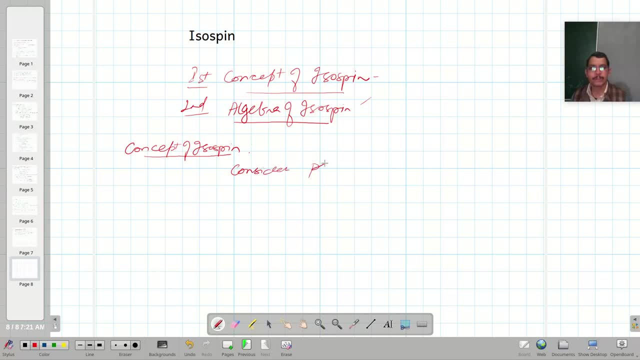 neutrons, Protons and neutrons. Let us have a look at their masses. So mass of proton is equal to 1.67262192 minus 27 kg, Whereas the mass of neutron can be written as 1.6749747 into 10 raised to the minus. 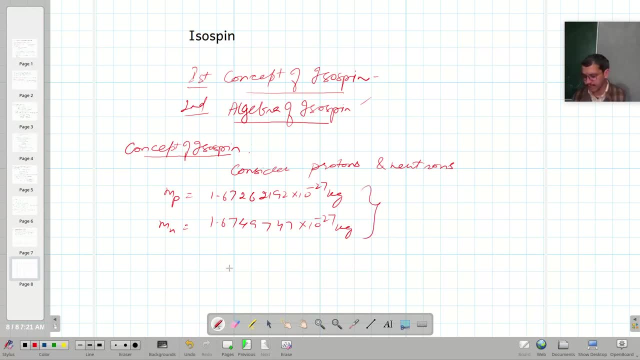 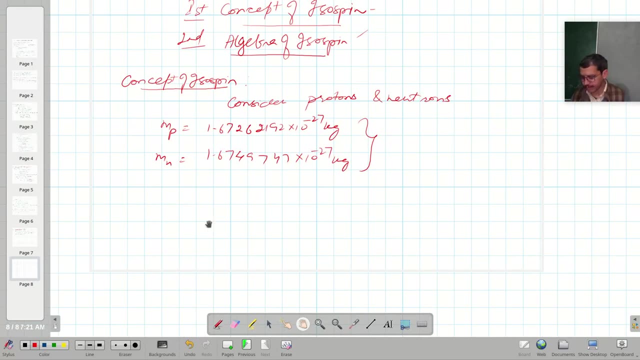 27 kg. So these are their masses And they are slightly different. Another thing regarding neutrons and protons is that nuclear force is responsible for, for stability of nucleus- right stability of nucleus- and this nuclear force is independent of charge. this nuclear force is. 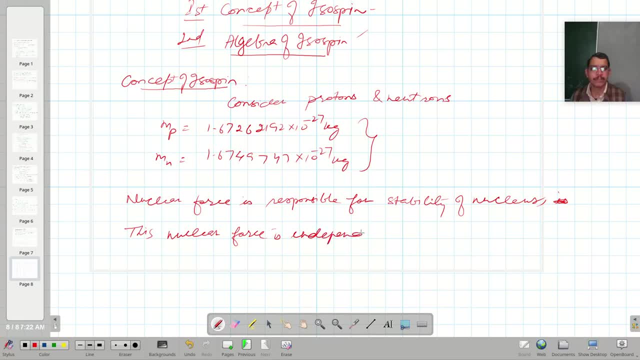 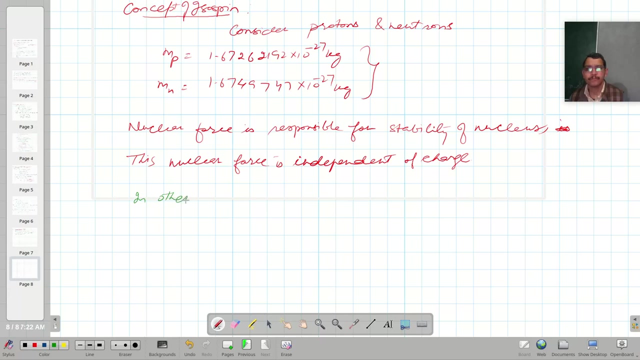 independent of charge. so in other words, we can say that we can say that strong force potential is same for all nuclear pair, is same, almost same for all nuclear pair. that means that means potential between proton and proton is nearly equal to potential between neutron and proton and potential between 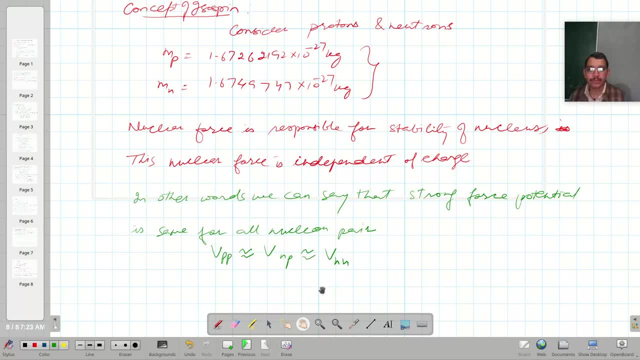 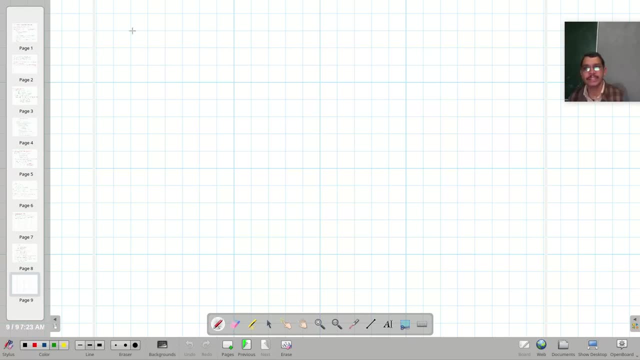 neutron and neutron. so Heisenberg, keeping all these things in mind, Heisenberg suggested that if we switch off, if we switch off electric charge of proton, electric charge of proton, if we switch off electric charge of proton, then we can say that if we switch off electric charge of proton, 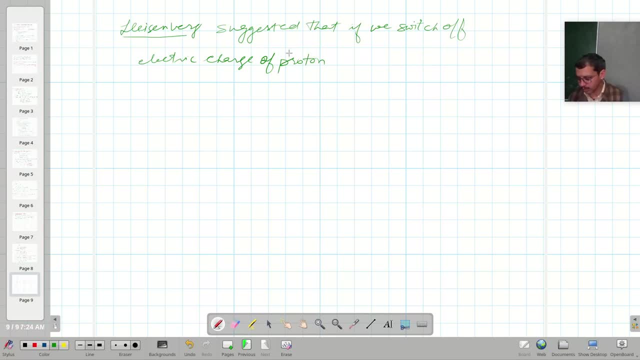 then we can say that if we switch off electric charge of proton, switch off lactic charge of proton, then we cannot distinguish between proton and neutron. right, we cannot distinguish between proton and neutron. so, keeping this in mind, keeping this in mind, it was proposed that it was proposed that neutron and protons are. 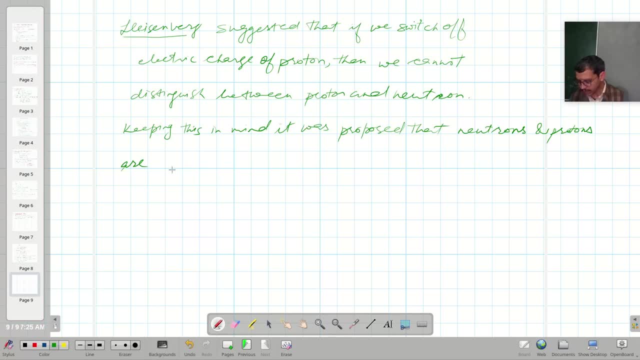 it was proposed that neutron and protons are true states of single entity, right, single entity, and it is analogous to, which is analogous to spin up and spin down, spin down states of states of spin half particles. so that means proton is represented by one zero state and neutron is 0: 1 and this leads to introduce, this leads to introduce the concept of 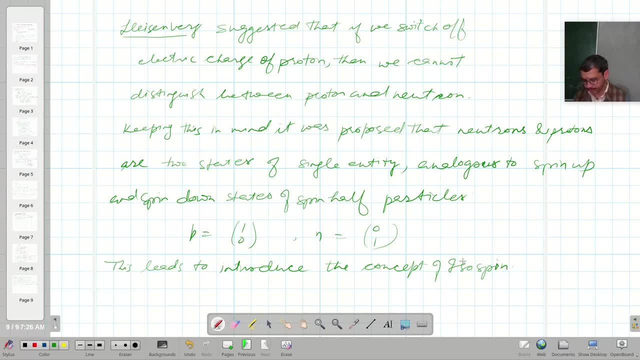 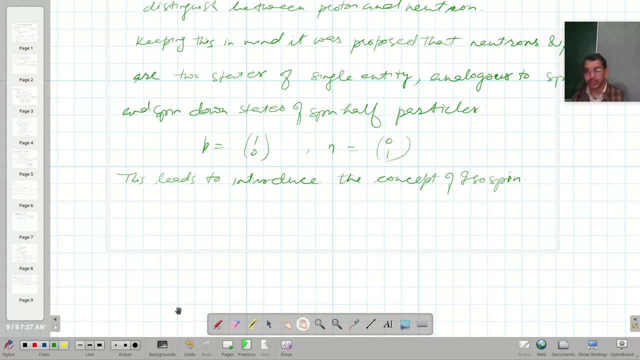 iso spin. so that means protons and neutrons, that means protons and neutrons. protons and neutrons form from protons, and neutrons form iso spin, doublet, doublet, and this is similar to spin with total iso spin. with total iso spin, i equals to. 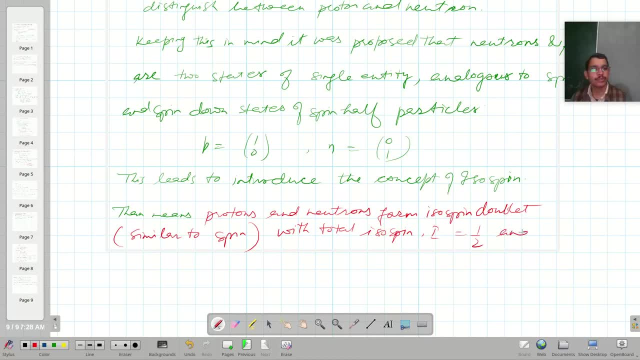 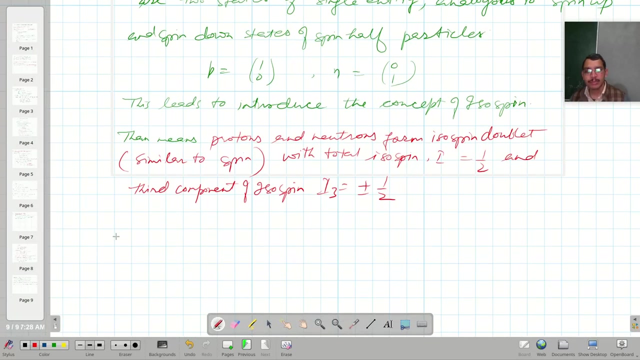 iso spin and third component of iso spin and third component of iso spin, that is i3, is equal to plus minus 1 by 2 for the proton and the neutron. so charge, independence of, so charge, independence of, And important thing is that the charge- this is very important point- charge independence, independence of strong nuclear force. 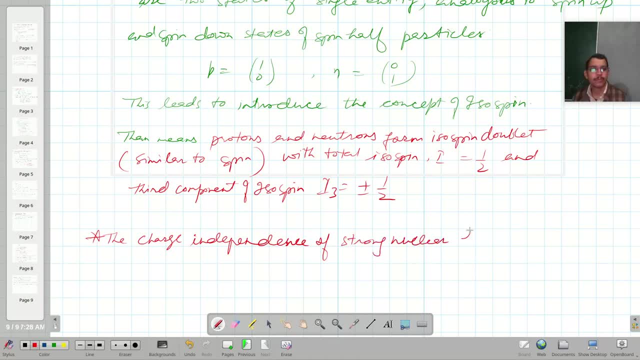 strong nuclear force is then expressed in terms of is then expressed in terms of invariance. invariance Under unitary transformation, under unitary transformation in the form of isospin space, in this isospin space, in this isospin space right. 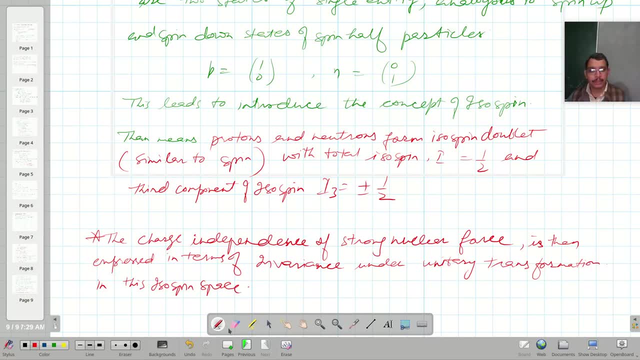 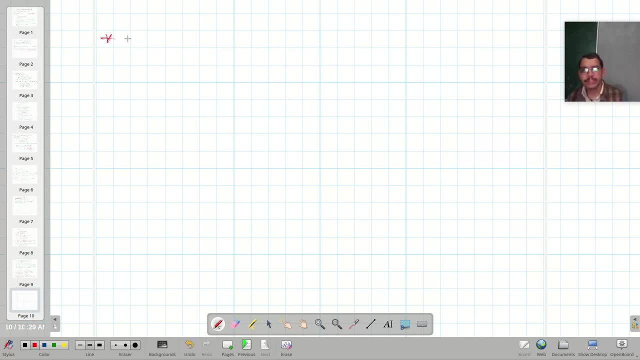 Right, Right Isospin satisfies. another important thing is that that isospin satisfies SU2 algebra. SU2 algebra- this is similar to SU2 algebra. Isospin- this is similar to spin. physically, isospin has nothing to do with the spin has. 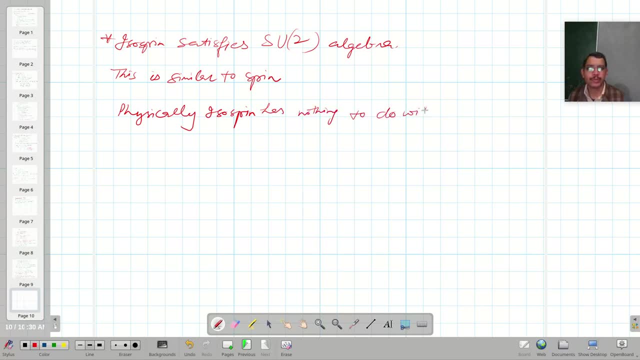 nothing to do with spin. Right Right Now, let us talk about the algebra of isospin. algebra of isospin, Like ordinary angular momentum, as we know that in case of angular momenta we have defined some rules. 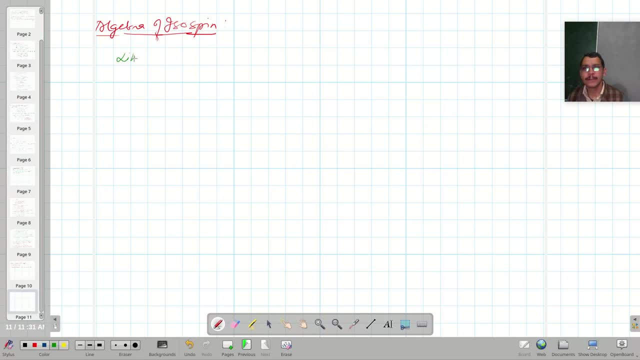 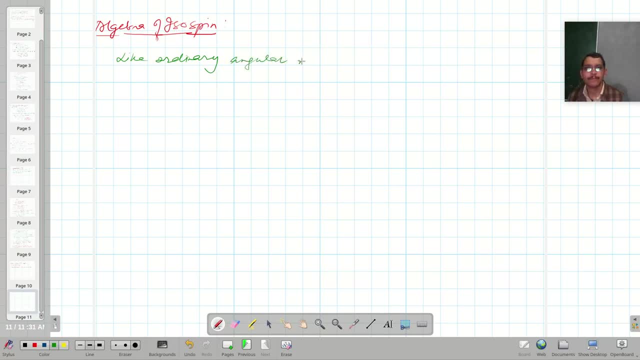 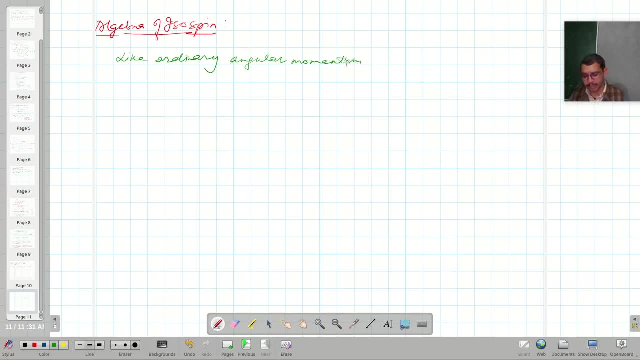 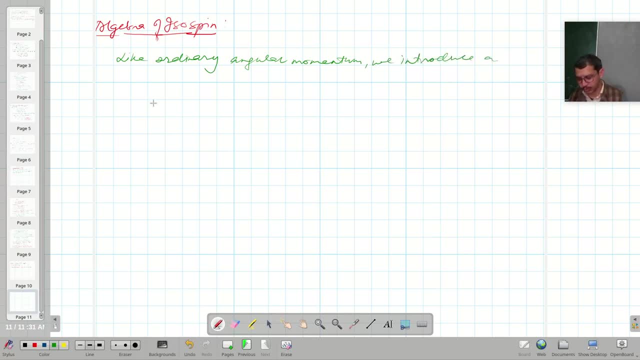 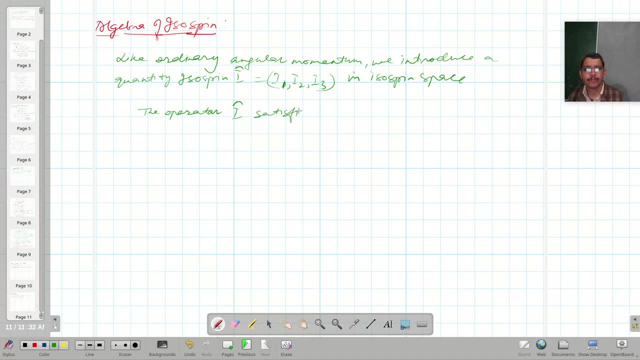 satisfies, the, the commutation relation of satisfies, the commutation relation of angular momentum, angular momentum, momentum j. so flow, keeping in mind the results of angular momentum, keeping in mind the results of angular momentum, let us define momentum, let us define raising, and define raising and lowering, and decreasing, and. 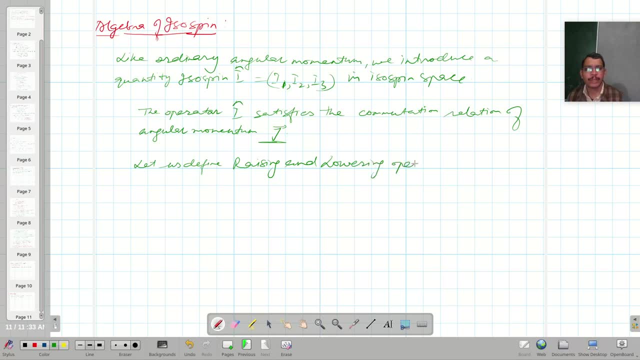 and loading operator for isospin space. So I call it as: I plus is equal to I1 plus Iota I2. and similarly I can define: I minus is equal to I1 minus I plus minus Iota I2.. This is called raising operator and we call it as the loading operator as we have defined for the case of the. 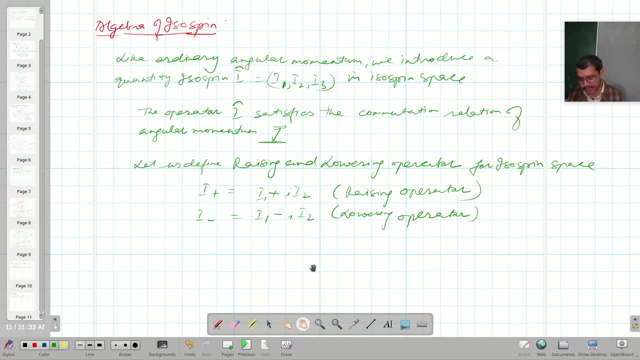 angular momentum also, It is similar to that- and matrix elements of the matrix elements of four isospin operators. So all these operators regarding angular momentum I talked about in the lectures of the quantum mechanics, So you should go through that. So the matrix elements of 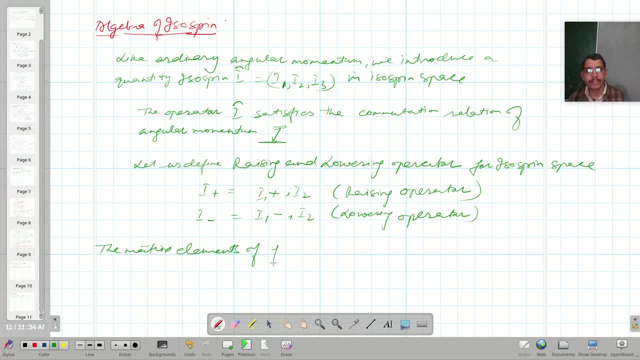 four isospin operators. four isospin operators, that is, I2, I3, I plus and I minus. with respect to, with respect to I comma, I3 as a basis are given, y as a basis are given by, are given by. so first is: 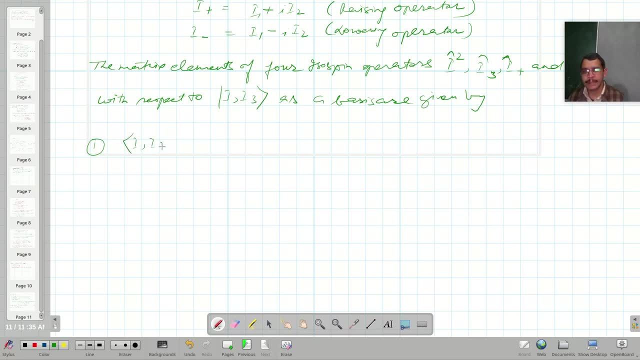 that is I, I3, I, I3, I2, I, I3, I2, I3 means expectation value of I2, means expectation value of I2 when operated in I3. it can be I into I plus 1, delta i3, i3, prime right or in some text it can be written as i square i- i3. it can be written as: 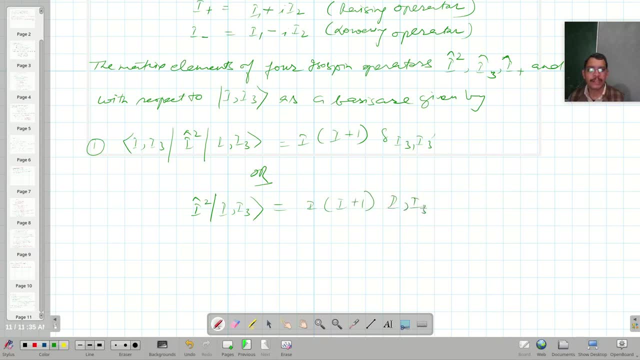 i into i plus 1 i i3. right, so one and same thing. then. second, is i i3, it's prime, it is i3, it is i i3, so it is i3 as it is means eigenvalue of this. i3 is i3, the eigenvalue of i square. 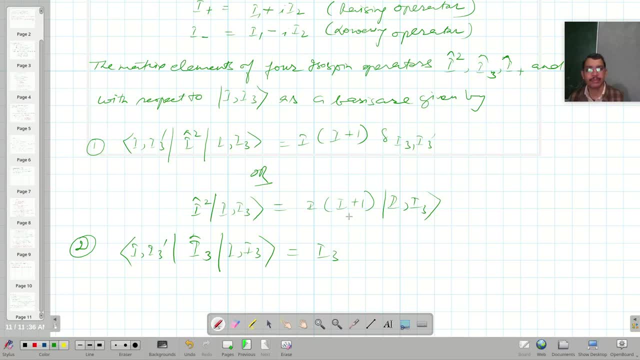 when operated with this i and i3, then it is i into i plus 1, so its eigenvalue will be this one and its eigenvalue will be this one, so it is i, i3- sorry, it is delta i3, i3, prime, or we can write it as: either we can write down: 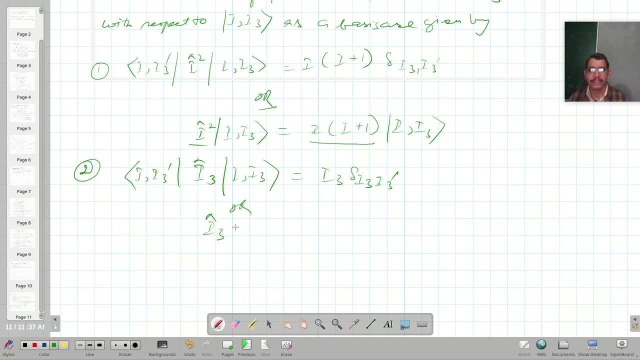 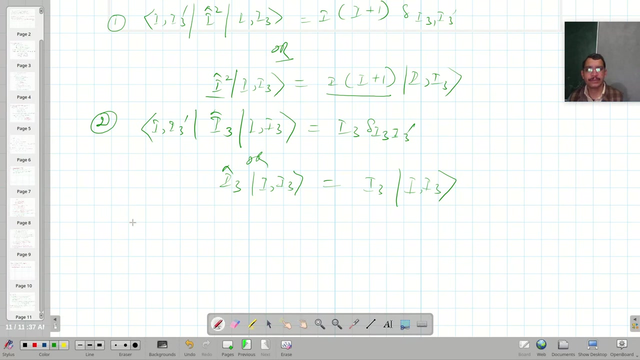 it as i i3- i3 or we can write it as i i3- i3 it this way or another way, is this that i3 i i3 is equal to i3 i i3 right? and third is very important thing which we have to keep in mind. this is very important. let me write. 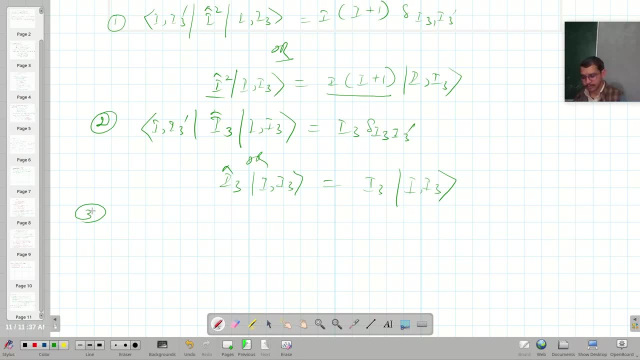 down there. so it is a i comma, i3 prime, i plus minus. for letter operator this relation is i: i3 plus minus 1. it must be equal to i into i plus 1 minus i3. i3 plus minus 1, whole under the root into delta: i3. i3 plus minus 1, or it can be also be written in some text as i plus minus. 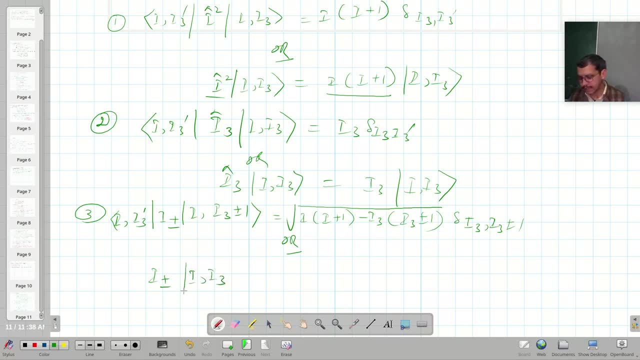 i i3 is equal to i into i plus minus 1 minus i3. i3 plus minus 1, whole under the root and multiplied by ket i i3 plus minus 1. so that's it like. these are the few relationship which we have to. 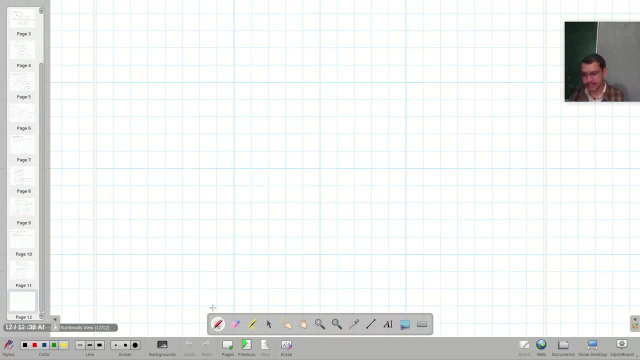 keep in mind the fundamental, two-dimensional representation of the fundamental, the fundamental, the two-dimensional representation of representation of isospin rotation group. rotation group is based on three matrices: matrices that is top 1, it is 0, 1, 1, 0 and these are similar to poly spin matrices, right. so 0 minus iota. iota 0. 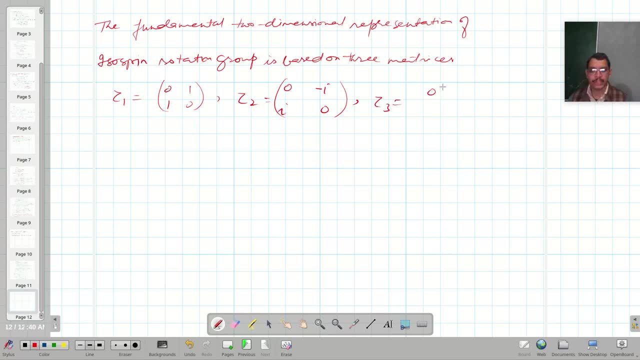 dot 3 is equal to 1, 0, 0 minus 1, so which are identical to poly spin matrices. which are identical to poly spin matrices also i. i can be written as 1 by 2 tau i, such that tau i y 2, tau i y 2. 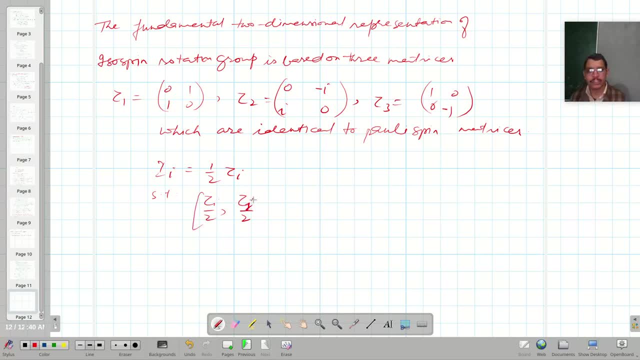 so their commutator- sorry, it is j tau j y 2. its commutator is equal to: i, epsilon i j k, top k by 2 and, keeping this in mind, we can write down it as i i i j. its commutator is equal to. 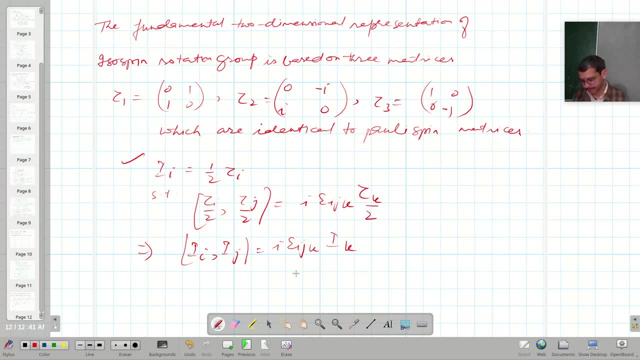 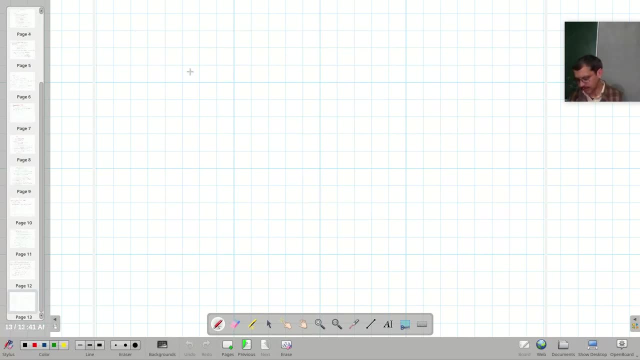 i, j, k, i k right. also i 3 has i 3 has 2, i plus 1 eigen states that is minus i 2 and so on. plus i in step of 1. possible eigen values of i are possible eigen values of i are: 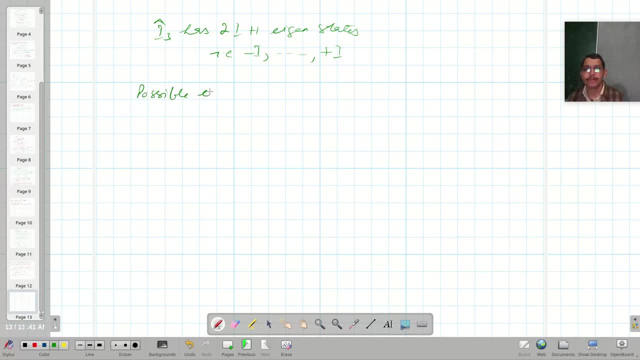 possible eigen values of i are amazing. they're either 0, 1 by 2, 1. they're either 0, 1 by 2, 1, 1, 3 by 2 and 2, and so they're either 0, 1 by 2, 1, 1, 3 by 2 and 2, and so. 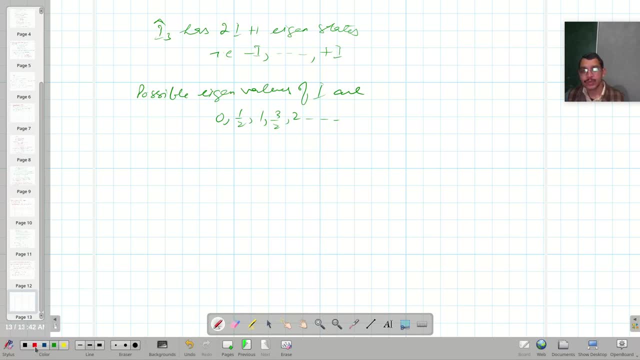 for proton. let me talk about this for the proton and then pilgrim. so for proton and for node neutron. let us talk about it, for proton is represented by p, get p, so it has. these are the values of the isospin, total isospin, and its z component. so it is 1 by 2 and 1 by 2. 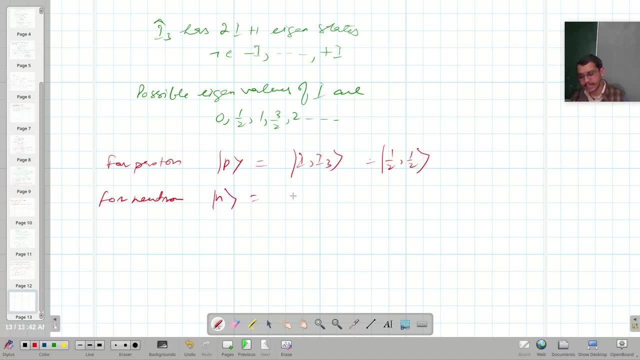 for the proton, but whereas for neutron it is 1 by 2 and minus 1 by 2, and similarly for pion. pions i i, 3, get i i 3 are given as. pion i i- 3, get i i 3 are given as: 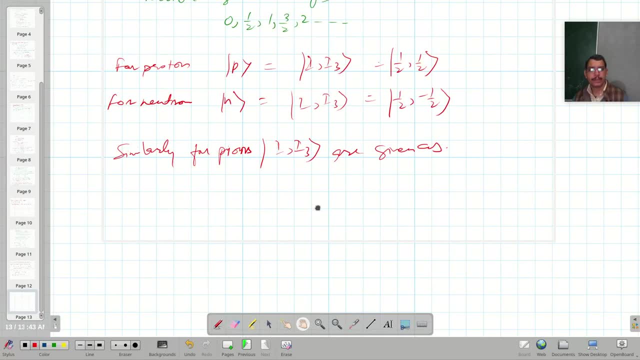 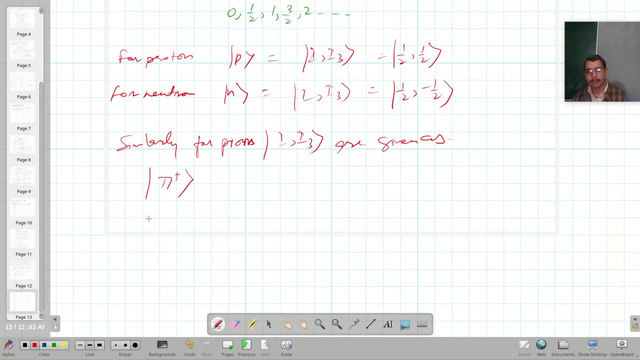 pion i i 3 get i i 3 are given as. let me write down. so for pi plus or pi naught or pi minus, we can write down the value of this state factor. it is 1: 1. it is 1: 0.